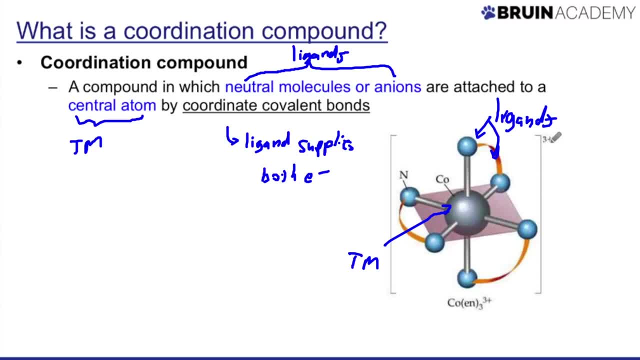 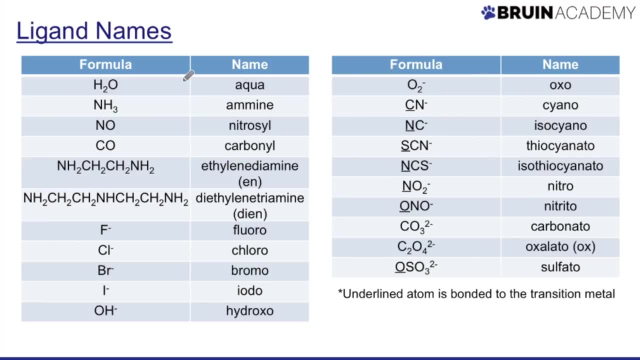 creates this sort of octahedral shape, And the overall charge of the coordination compound is plus three. All right, So like that VSEPR theory, I would have to say that there's a lot of memorization for coordination chemistry, And I think the best way to do this is flashcards. So on the left hand side here you see the formula And on the right you see the name. This is something you have to memorize. You won't be given this on an exam. 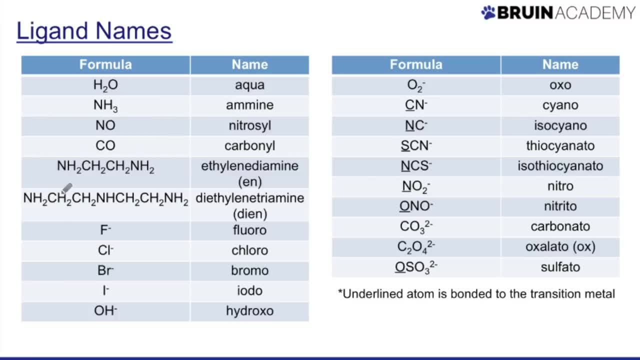 So let's go to the next slide. Notice that some of these ligands are neutral. So these first guys are neutral And then when you hit some of these halogens they have a minus one charge. And then all these guys- a lot of them- are polyatomic ions. They have negative charges of either minus one or minus two. I would say that the easiest way to learn coordination chemistry is just to practice and do problems. At first you should have these tables in front of you. I would say, after a while you should try to do these problems without the tables. All right, So let's go to the next slide. 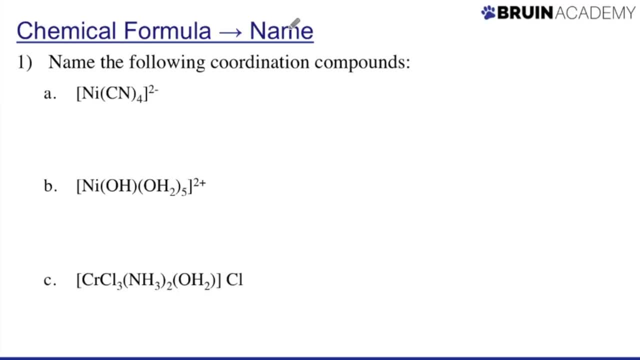 from chemical formula to name, which I think is actually a bit easier than the reverse. so we're going to start with a formula and we're going to give it its name. so going to start with nickel and we have this CN for them and the overall charge is two minus. so the easiest way to go about this is to start. 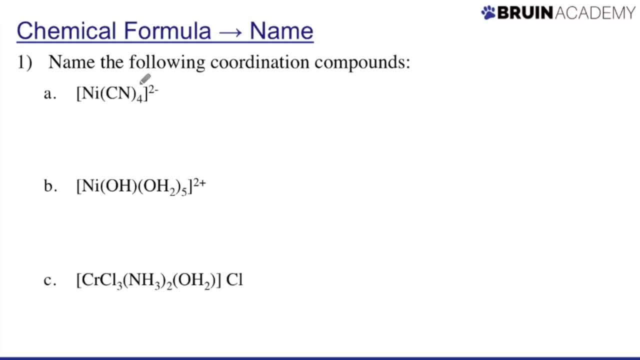 with what's in the brackets here in some of these. in this first example, there's only one guy in the brackets here in Part C, we have something in brackets as well as something outside of brackets. start with what's in the brackets. what's in brackets represents the coordination compound. so this is your coordination. 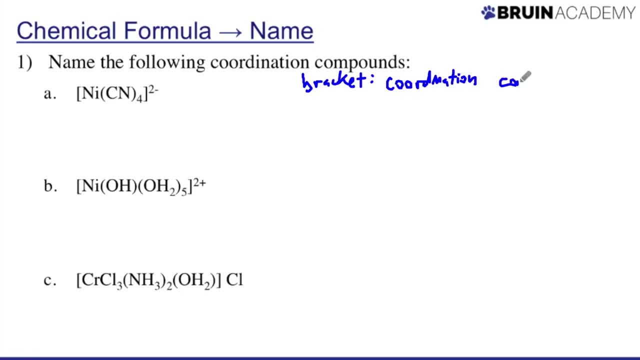 compound, and you can probably already guess which one is going to be a ligand and which one is going to be the metal. right, the metal is the nickel. when we name coordination compounds, we start with the ligand. so this CN is called a cyano group. I have four of them, so I call that tetra cyano and then I write: 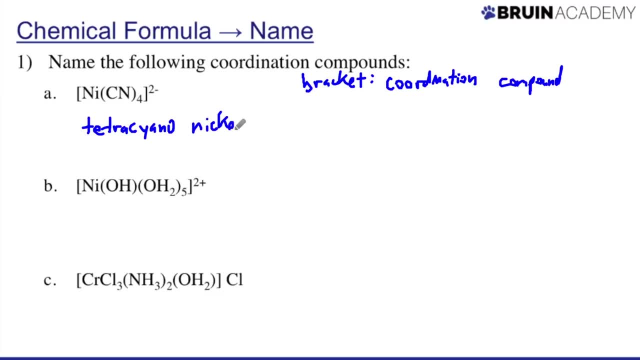 my nickel right. so because the overall charge of this is a minus two, it's an anion, and so whenever it's an anion, you write eight at the end, instead of just writing nickel, I write tetra cyano nickel eight. I'm not done because I need. 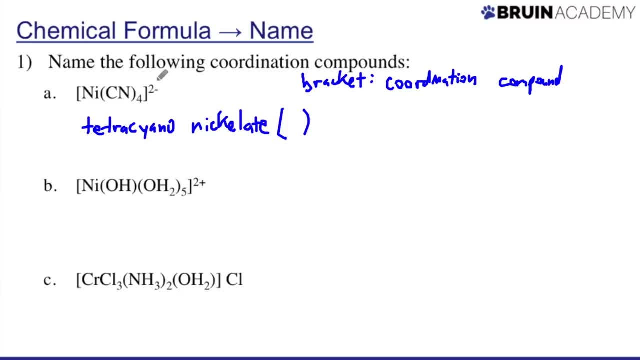 to actually specify the charge of my nickel, and I can figure that out fairly easily, because I know that cyano has a minus charge of one minus one charge. I have four of them, so the cyano is minus four for the four of them. and so, in order to make it, this entire thing in brackets- 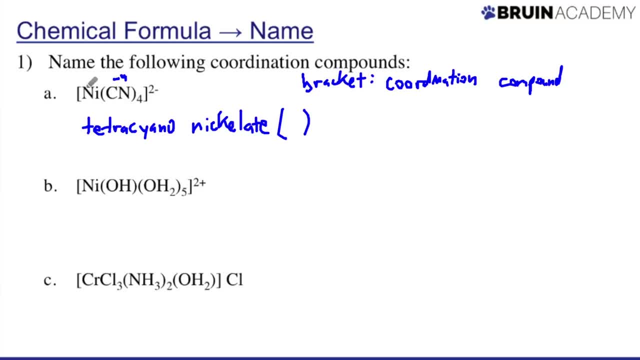 have a total charge of minus two, my nickel. it needs to have a charge of plus two right, because a positive two minus four is a negative two, and so I write in bracket, in these parentheses, real minimal two right, and so I can do the same thing for B. so I start with the ligands which are in this parentheses. 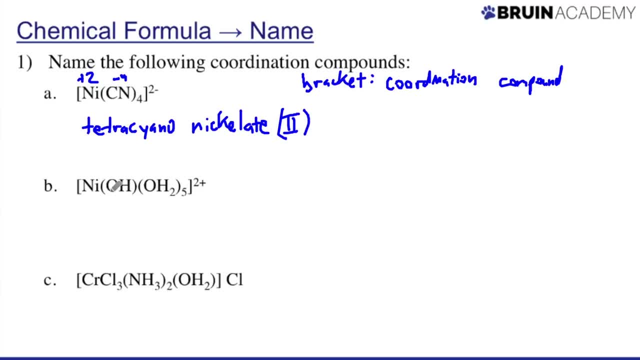 and I always name an alphabetical order right. so the OH is a hydroxyl group, the OH two, in other words an H 2 O, is a, an aqua group, and I write that first. I have five of them, so I write penta aqua. 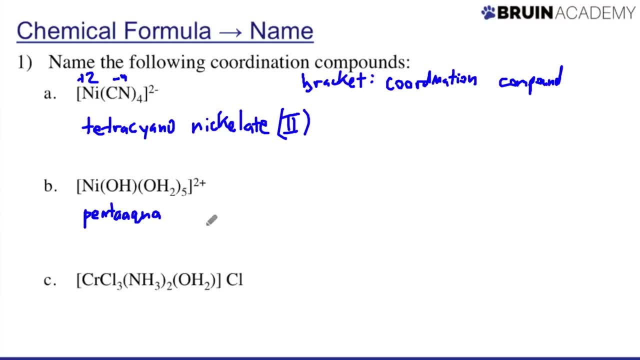 and then I write hydroxyl, because H becomes comes after a, so I write hydroxyl next, I just have one of them, and then I go ahead and write nickel. so here the overall charge is not a negative, instead it's a positive. and so what I'm gonna write is nickel. I'm not gonna need the eight, I'm just gonna. 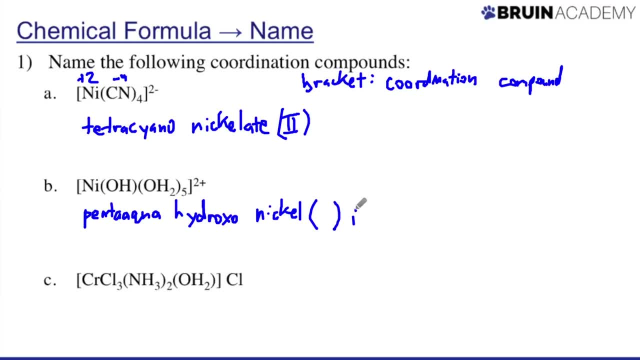 write nickel- I'm gonna save for room for the charge and then ion. so whenever it's an overall positive charge, you just write ion at the end and now we have to figure out what charge the nickel has, right. so hydroxyl has a charge of minus one, right? this is something you get from. 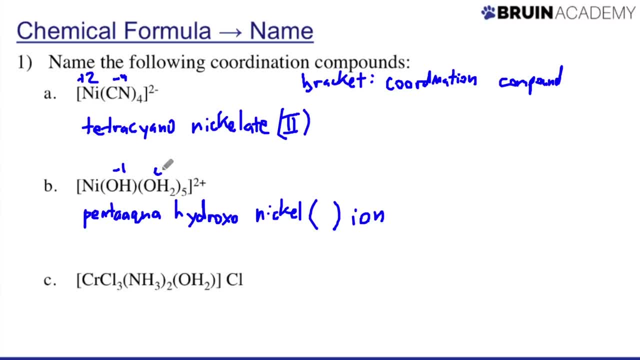 the table water is neutral, aqua is neutral, and so in order to make this overall coordination compound having a charge of two plus, the nickel needs to have a charge of three plus, and so then I write nickel three ion, all right. and then this last example: okay, so we start with what's in the parentheses, that's: 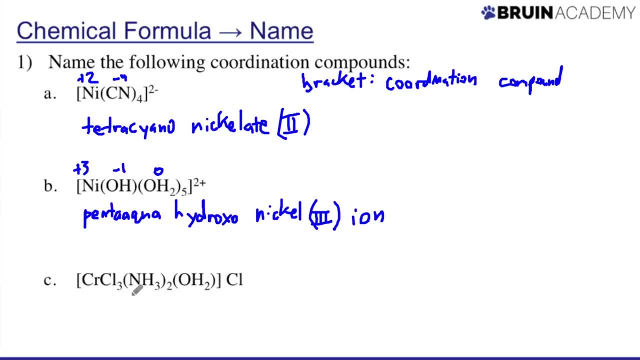 inside the brackets. that's the coordination compound. I name things in alphabetic order. so here I have a chloro group, I have an amine and I have an aqua. amine comes first. I'm going to write di-amine, because I have two of them. 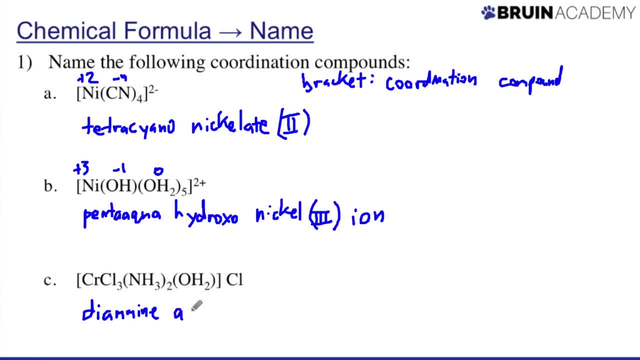 I have one aqua, so I write aqua and then I write tri-chloro, because I have three of those guys, and then chromium, and then now i have to figure out the charge of chromium right, and so notice one thing here is that i have a chlorine after right before i had actually charges and nothing. 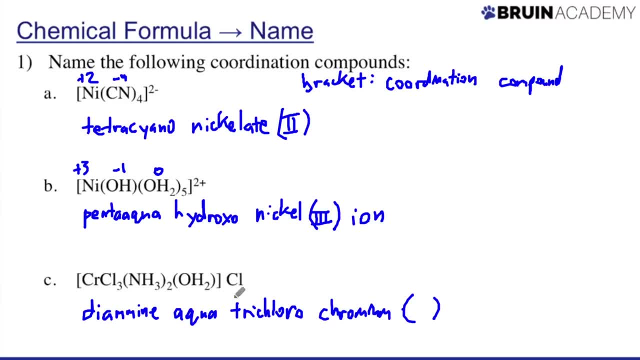 attached. here i have a chlorine and the chlorine is going to be an anion. remember, it's one of the halogens. it has a minus one charge whenever it's an anion. instead of writing chlorine, i write chloride, right. what that tells me is that the overall charge of what's in the brackets has to. 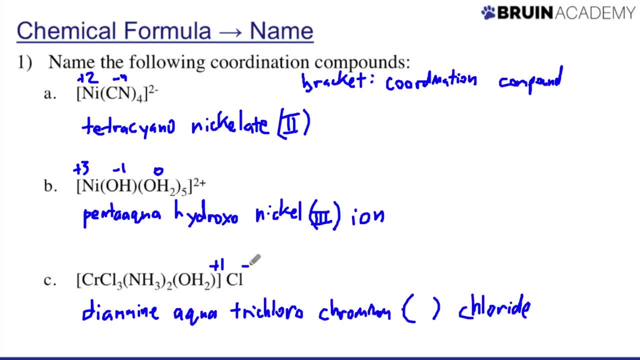 be plus one, because i know that the chlorine has an overall minus one charge and overall this thing is neutral right, and so i can figure out if this is the total charge of plus one. i can figure out the charge of chromium right. chlorine is minus three because each one is minus one and i have 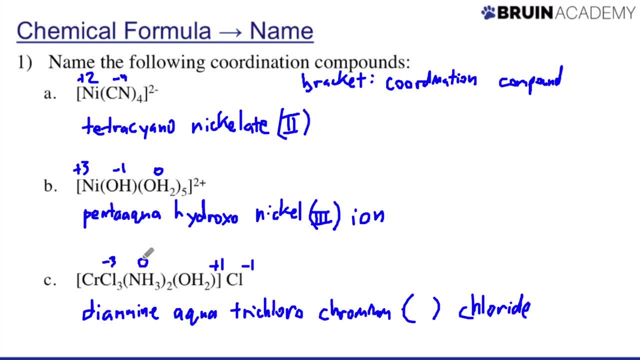 three of them, amine, is neutral, and so is water right. and so if my overall charge is plus one, what charge does chromium have to have? it has to have a charge of plus four, and so i write chromium four chloride, and here i don't need an ion, the word. 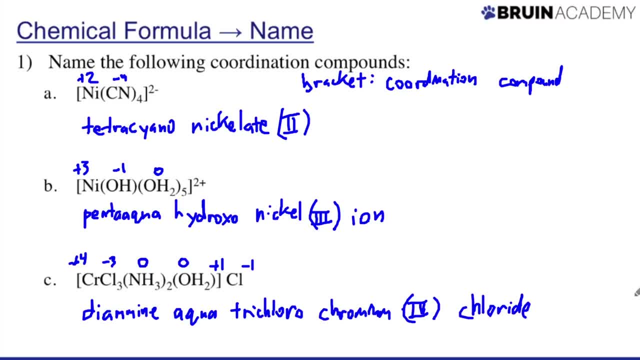 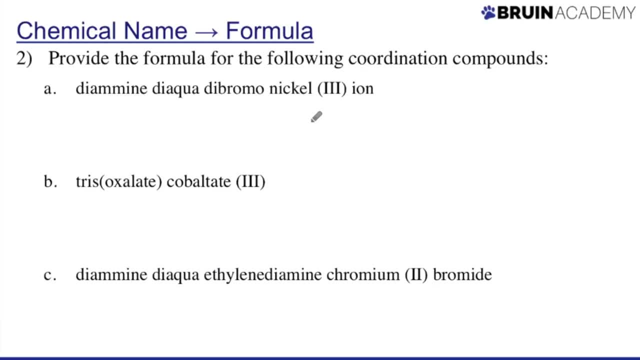 ion after chromium, because i have the chloride, the chloride after that. so the second way that you'll be asked these types of questions is to be given the chemical name and write the formula right. so i think this is a. It's slightly more tricky, but it's the same logic, right? 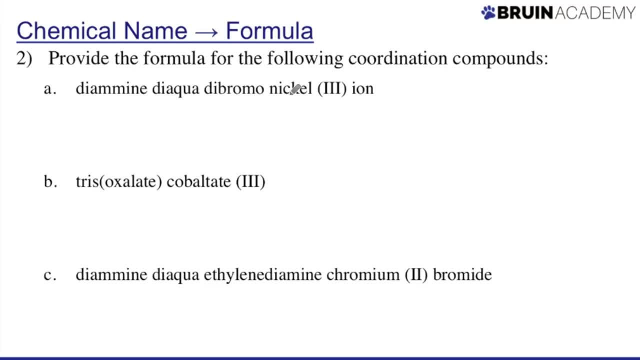 So we'll start with di-amine, di-aqua, di-bromo, nickel-3-ion. So I start by writing out my brackets. I know that my coordination compound is what I write first. The transition metal is what I write first, so I write nickel. 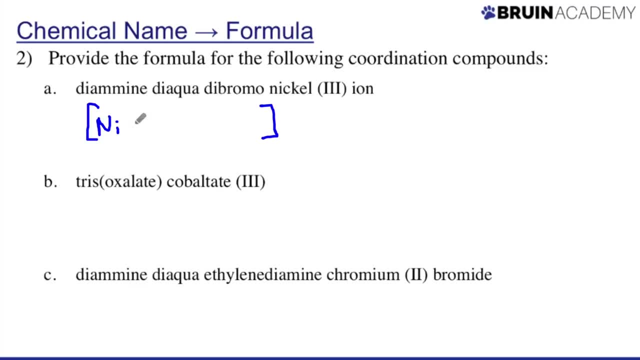 And then I write my ligands in parentheses, And so the first one is amine. I have two of them, So amine is NH3, and I have two of them. I have two aquas, so that's H2O. 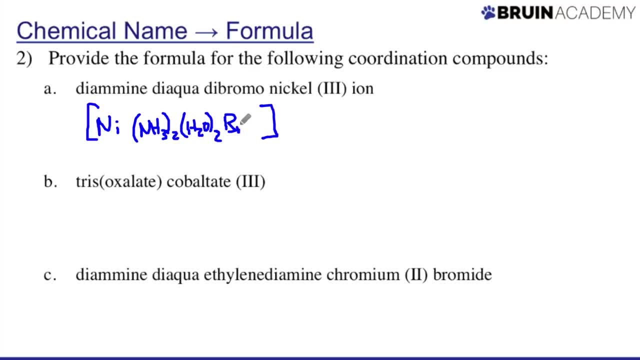 And then I also have two bromines, so I'm going to write Br2.. The last thing I have to figure out is what the overall charge of this coordination compound is. So I know that nickel is plus 3.. I know that NH3, amine is neutral. 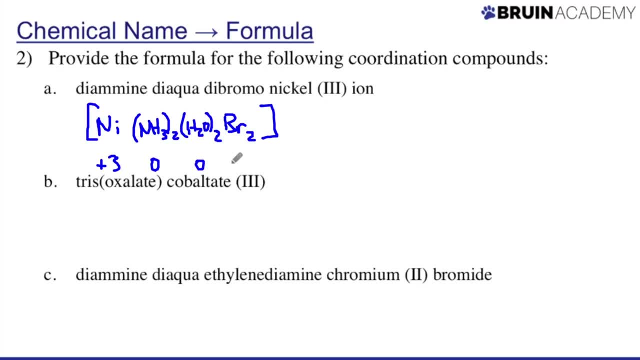 Aqua is also neutral, But bromine is minus 1.. And I have 2., So that's minus 2.. So positive 3 minus 2 is going to get me a positive 1 charge, And so that's the coordination compound as well as its charge. 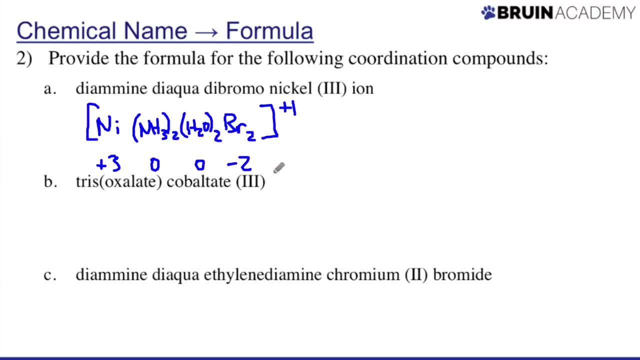 We can do the same thing for part B, So tris, oxalate, cobaltate 3.. So we'll start with our brackets and our transition metal, which is cobalt, And then here our only ligand is oxalate, which is- you can either write it as OX or 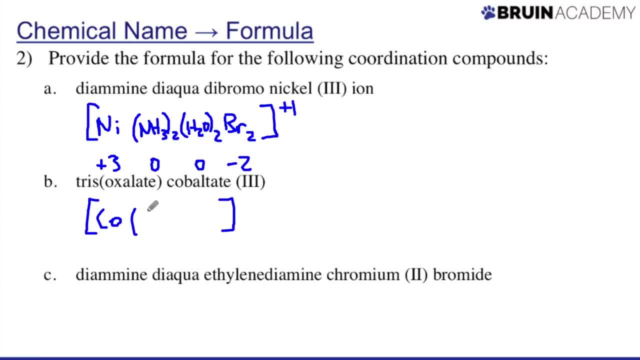 you can also write it as OX, So I'm going to write it as C2O4, again something you should memorize- And I have three of them, tris. So here you would say tri, but because there's a value, you add that S. So tris, oxalate. 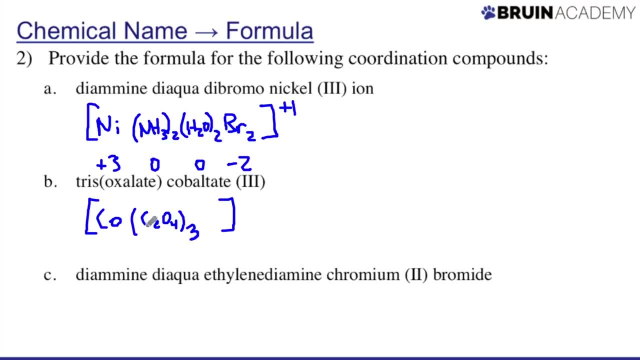 And I have three of them, And I know that the overall charge of C2O4, oxalate is minus 2.. I have three of them, so that's minus 6.. And then my cobalt has a charge of plus 3.. 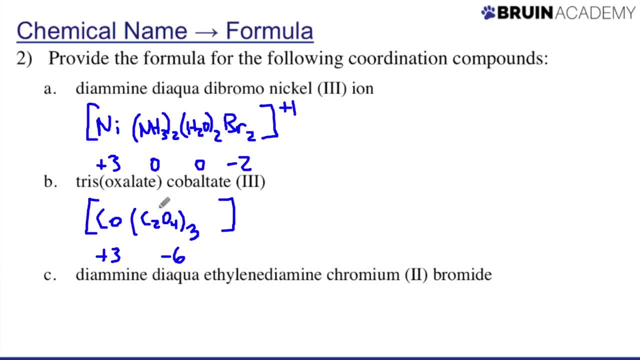 Because the Roman numeral is 3. And so my overall charge of this guy is going to be minus 3.. And that's why the 8 is here, because my overall charge is negative and it's an anion. Okay, so the last example: diamine, diaqua, ethylene diamine, chromium 2, bromide. 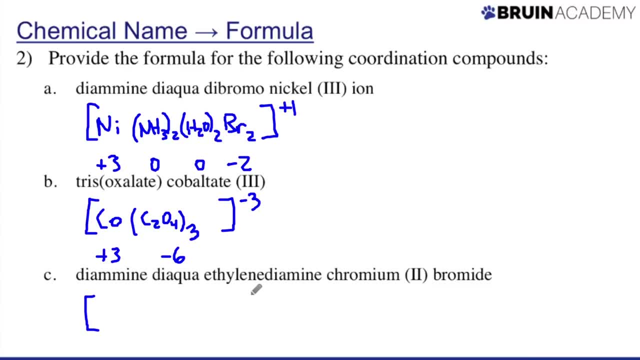 So we're going to start with our brackets. as always, Our transition metal is chromium, so I'm going to write chromium here And then I'm going to write in my ligands, Right? So the first one is NH3, amine. 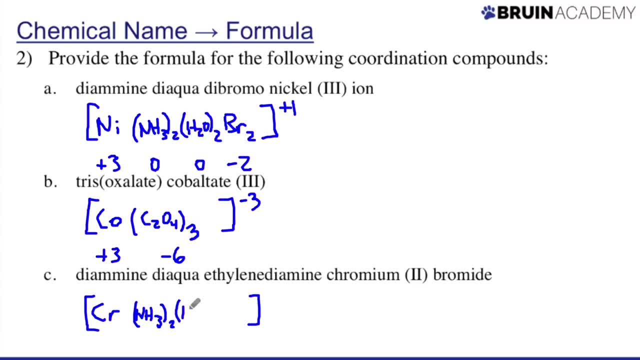 I have two of them. I also have two waters, so I'm going to write H2O2.. And then I have ethylene diamine, right, So you can actually just abbreviate ethylene diamine as EN. You don't have to write the entire structure that you saw on the table.